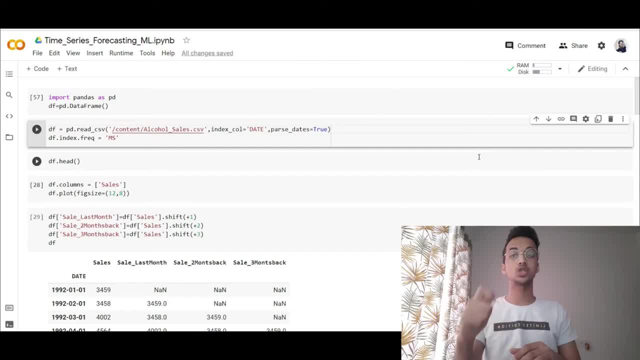 making predictions. In this video, I'm going to take a data set and show you how you exactly need to manipulate that so that you can use any of your ML models, like linear regression, random forest reversers or any regression model, in order to make a prediction. So I'm going to straight start. 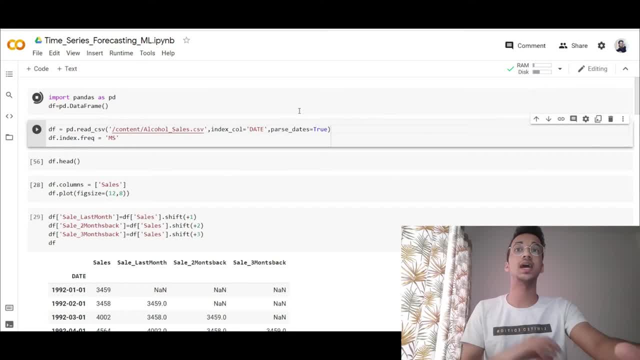 away with the code. right, I'm going to import pandas as pd and I'm creating a blank data frame. right now, I'm using a data set that contains data about alcohol sales for each one from 1992 to, I think, 2020.. I'm going to leave this entire code, as well as the data set in the description, You can. 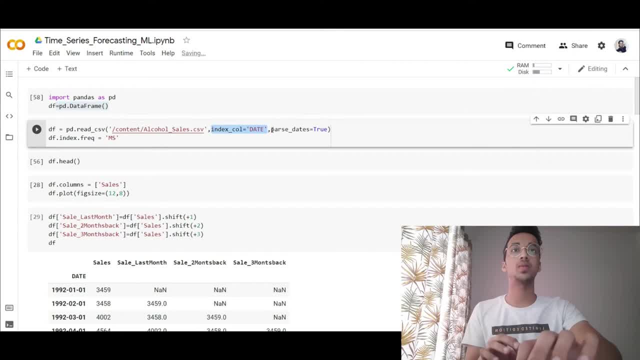 go through that and basically the index column is going to be date and I'm going to write: parse dates equals to true. Then my pandas data frame is going to be true. So I'm going to go ahead and I'm going to create it like a date and not just a random string. So I will just print the first. 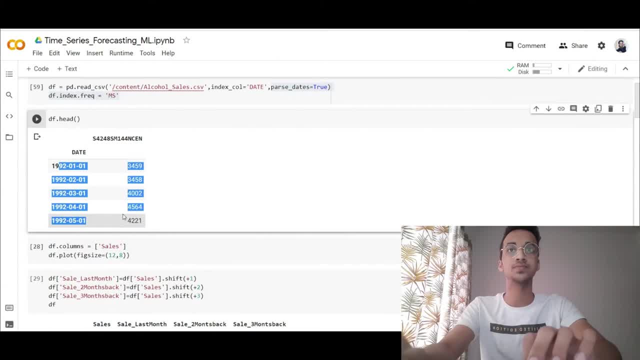 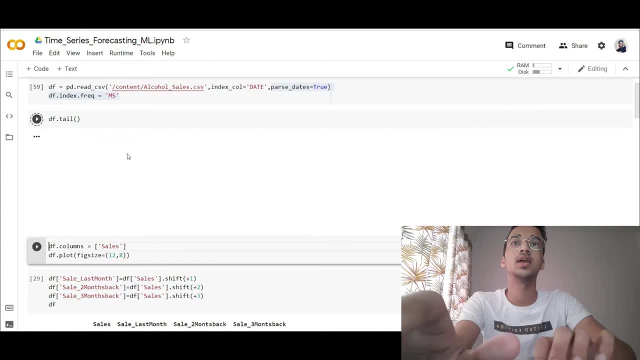 five values. You can see how it looks like. You can see I have monthly data right Of alcohol sales And I can also look at the last five values using dftail and it goes up to 2019.. So, in time series forecasting, you're going to have data like this. You're going to have a 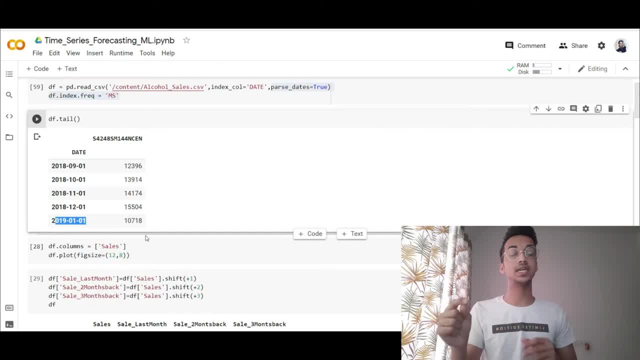 sequence of data. What you have to do is you have to convert this data to supervised learning. In supervised learning for machine learning, you have to convert this data to supervised learning. Right, You basically need to have an input and an output. You have to create that input and output. 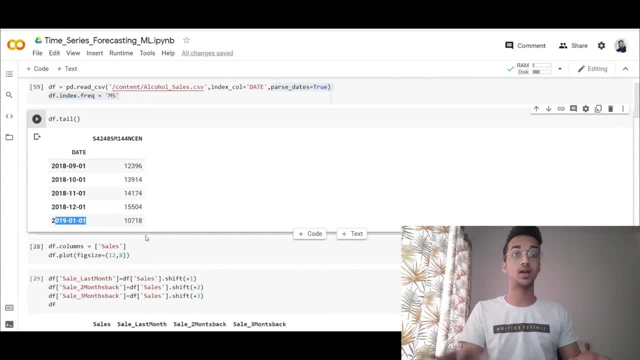 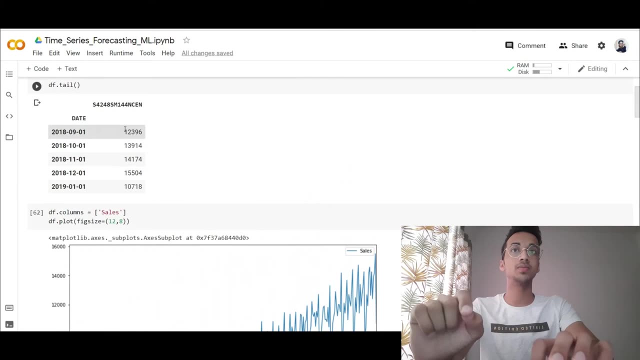 for it. Now I only have the input column, which is the time series. So how do I make an output column? That is what we're going to figure out for now. Let me just plot this data and this is how it looks like. So what do I need to do now? I have an input column. I need an output column in order. 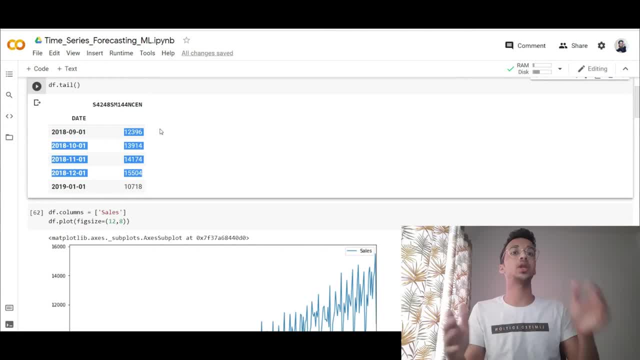 for my model to learn a relationship between input and output. For example, let's say I'm going to be using the past one month's value in order to make a prediction, Then what do I need So, for example, if I have this particular 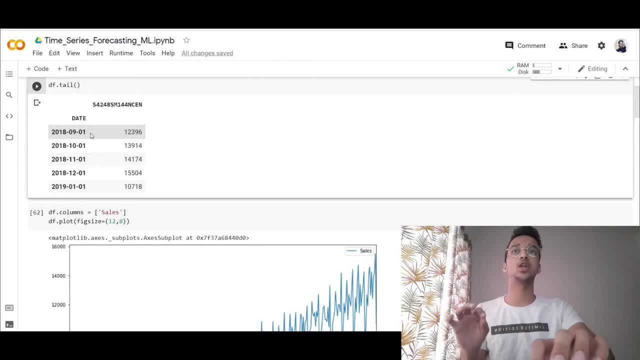 row as my input, which is, let's say, the data of 2018 and 1st September, then I need to make a prediction for what is the sale is going to be in the next month, in the month of October, right? 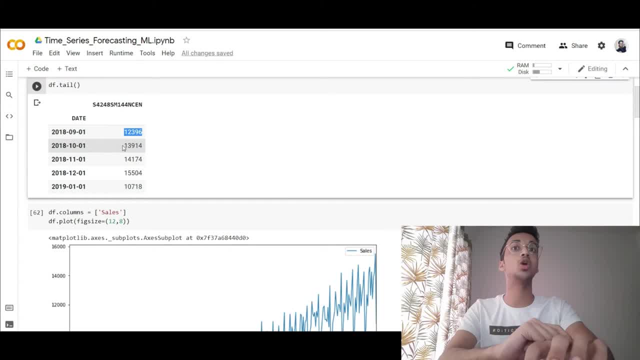 So if this is 1,, 2,, 3,, 9,, 6 is my input, then my output should be 1,, 3, 9,, 1, 4, which is the sales in the next month, right? So I just need to have another column. 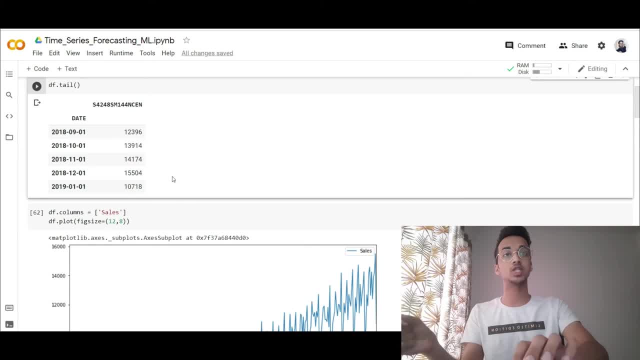 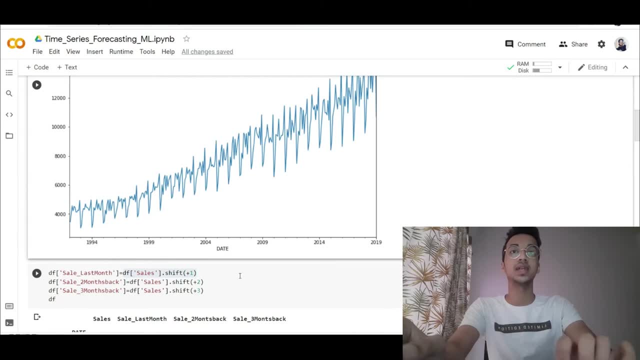 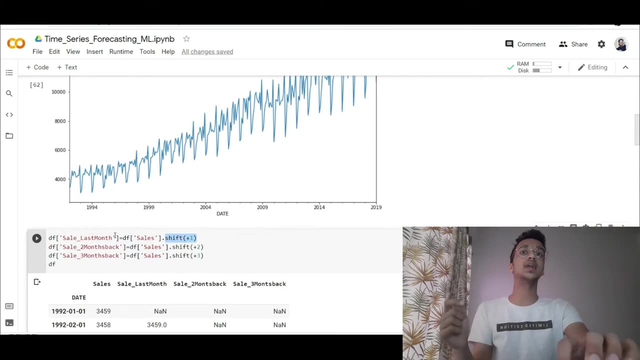 over here, which contains the sales in the previous month, which is going to be the input, And using that, I'm going to predict the sales in this month. To do that, I simply take my sales column and I shifted that by one unit, So, and I save that as sale underscore last month. So now, 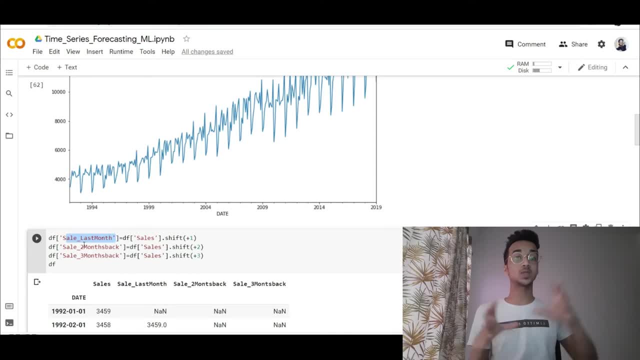 I will be using the last month To make the last month's data to make a prediction for today. But what if my data, but what if my current value also depends on the sales two months back or sales three months back? that is what you. 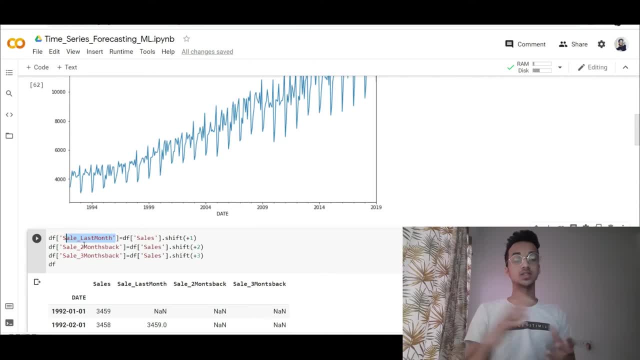 have to figure out. If your data has a repeating pattern every six months, then you might have to use the past six time period values. So I have made videos on using the PMD auto ARIMA functions as well, which will tell you what is the order in your data set, which basically lets you know how. many past values you have to use And what is the order in your data set, which basically lets you know how many past values you have to use. So I have made videos on using the PMD auto ARIMA functions as well, which basically lets you know how many past values you have to use And what is the Caption. 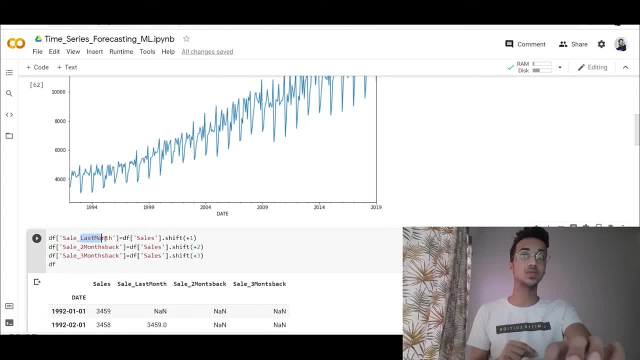 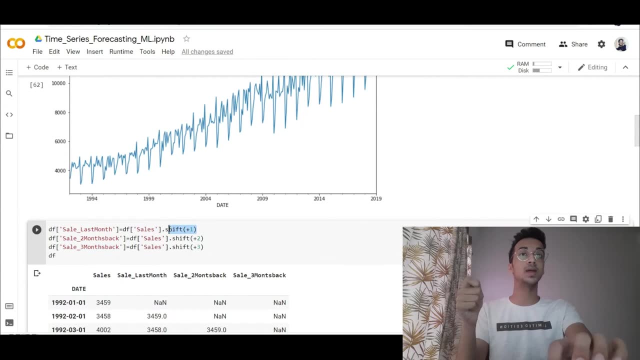 value. So for now I'm going to consider three values: the sales in last month, sales two months back and sales three months back. I simply get that by shifting that, shifting my sales column by one unit, two units and three units respectively. So when I print my data set you can look at. 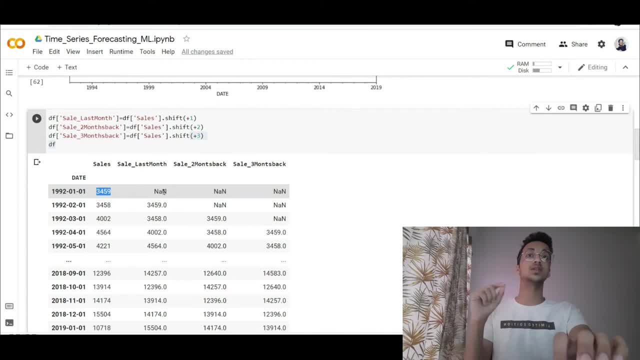 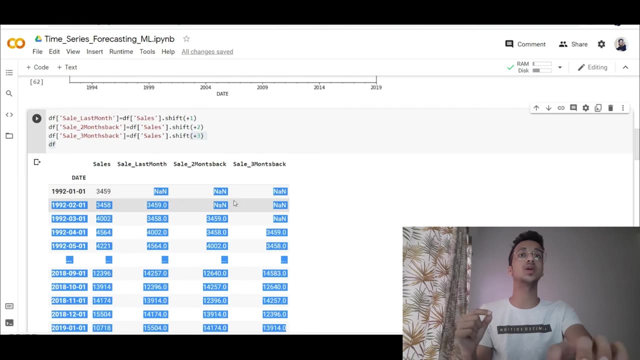 this. this is how it looks like. So for my first row, the sales in last month row contains any N value, which basically means not a number, because was no information prior to the first data right, so it will be as nan. similarly for two months and. 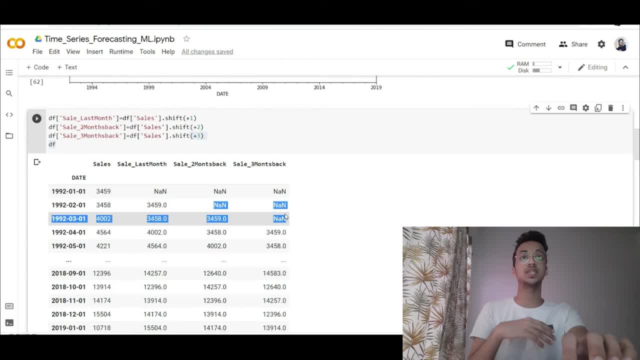 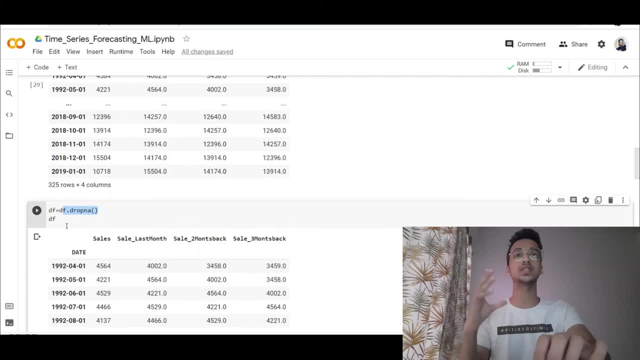 three months back, i will have this nan values, which basically means that they are invalid and i have to remove that before moving forward. so by using dfdropna, i'm gonna remove all those nan values and here is how my final data set looks like. so the sales last month, two months back, three: 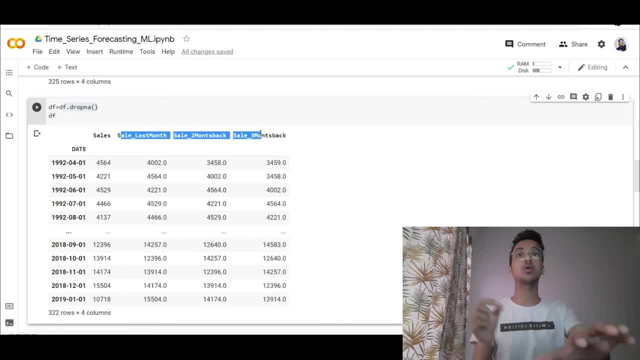 months back is my input column. using this input i'm gonna predict the sales in any given month, right? so my input and output is ready. now i simply have to call any machine learning model i want and give it to that. so i simply import the linear regression class from sklearnode: linear underscore. 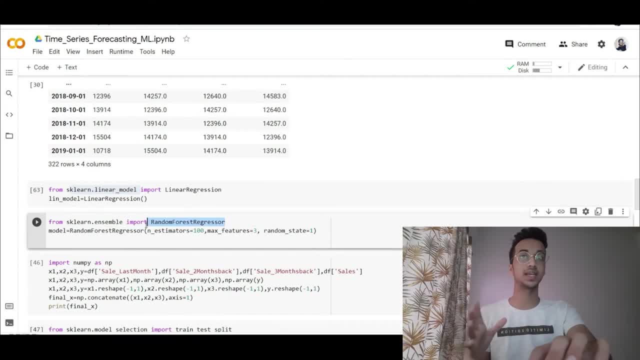 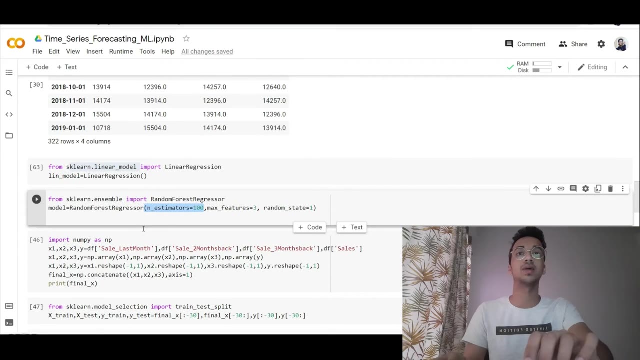 model and i also call the random forest regressor and i'm using some default values, which are normally work well, of max features equal to 3 and 100 estimators. so again, you can use any machine learning model you want and basically a regression model. that's all you have to keep in mind. 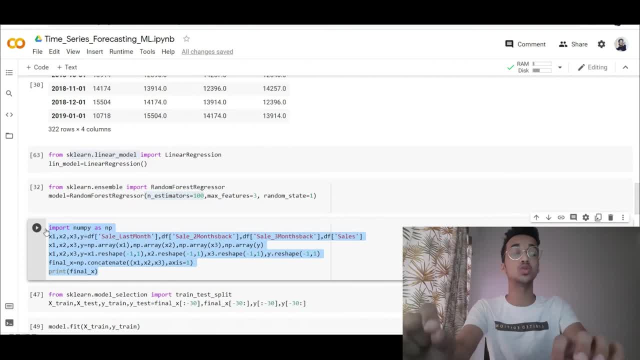 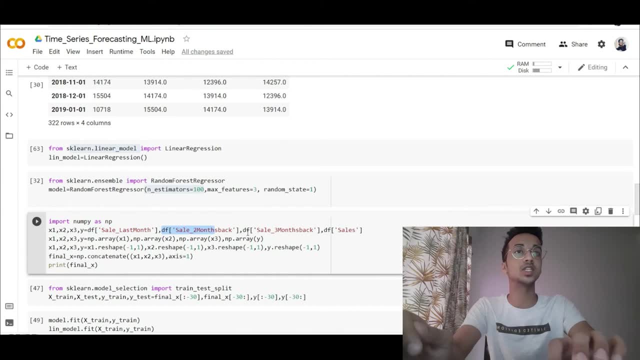 so here is a slight bit of data pre-processing that you need to do, and that is all. so, basically, i am extracting my sales in last month, sales in two months back and three months back, and i'm saving it as x1, x2 and x3, which are 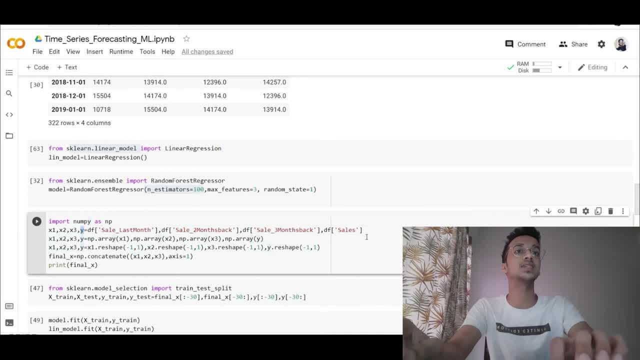 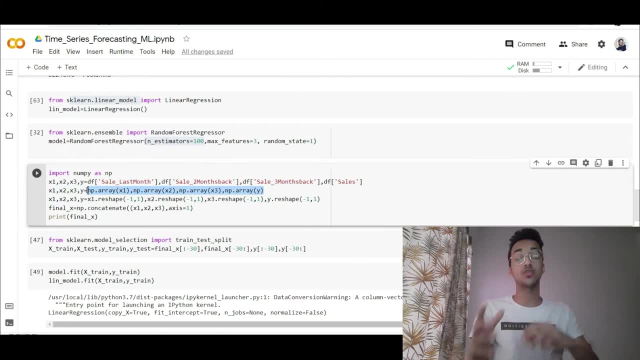 gonna be my input and the output column y is simply my sales, which is in the current month. now i simply convert all of them into numpy arrays. right, this is kind of necessary. you, i simply convert all those into numpy arrays and i reshape that into minus one comma one. so minus one comma one means we don't care about how many rows are. 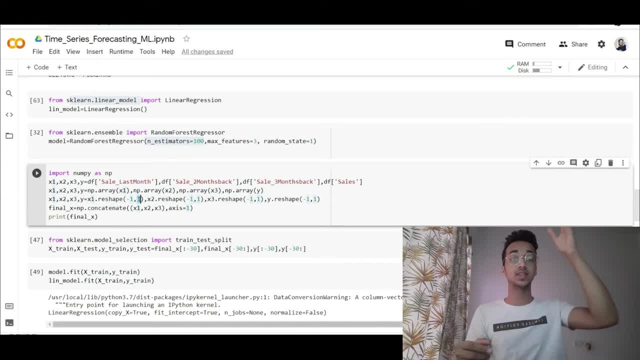 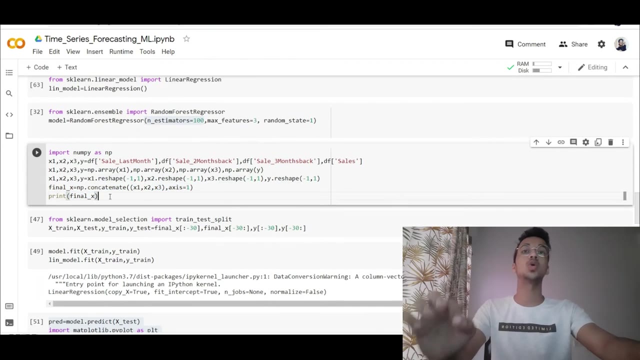 that is what minus one stands for, and this one means that there will be a single column. so i will have x1, x2, x3 as single columns and i'm going to concatenate them. so again, my final, x final input is simply concatenation of x1 comma, x2 comma, x3. so if i print my final output here, 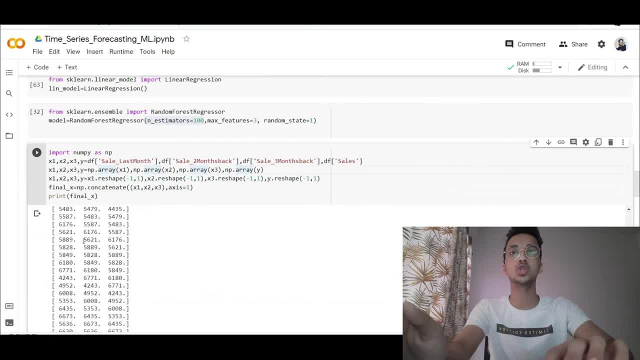 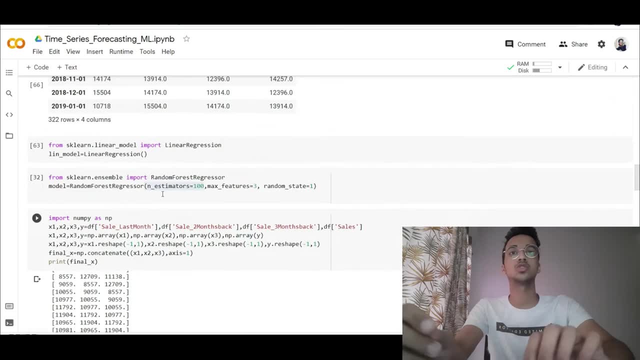 how it's look like, right, it's just a numpy array of three values which are my last, one months back and three months back value right, and it will use this to make a prediction for the current month. so now i simply have to split the data set into training and testing. i'm reserving 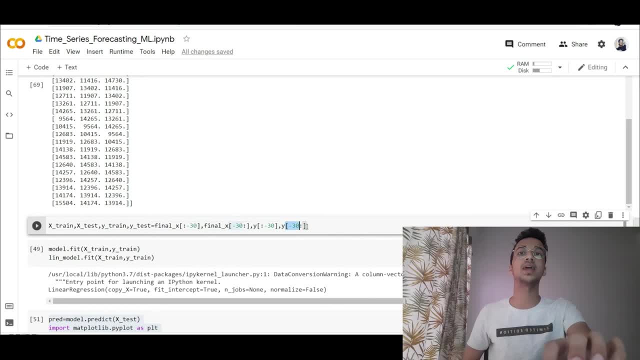 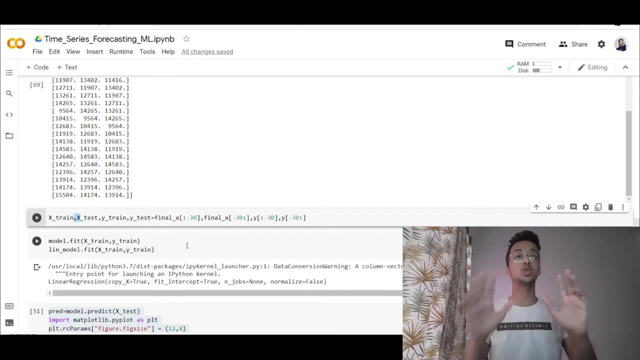 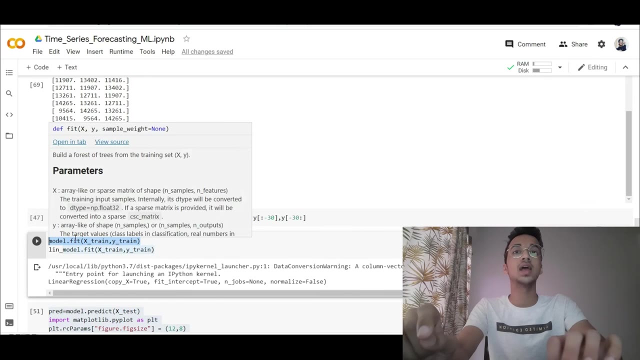 the last 30 values, as you can see, for my x test and y test, and the other values are going to be used for training. so over here i'm going to be using two machine learning models to show you in comparison. right, so i'm. modelfit basically stands for the random first model and lin underscore. 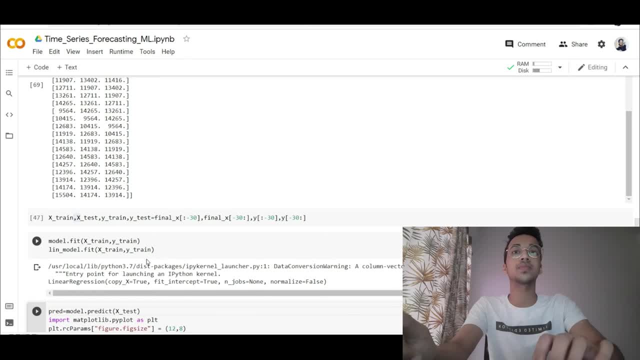 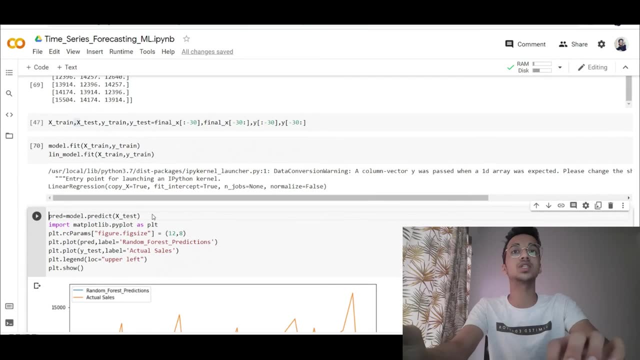 regression model. so i've fitted the model onto that data and now i'm going to make you, i'm i'm going to make the predictions and we're going to see how it works right. so to make the prediction, i first make predictions on the testing set. i import matplotlibpy plot, splt and i'm basically 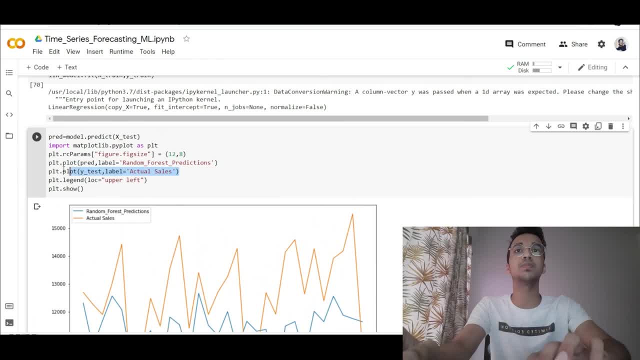 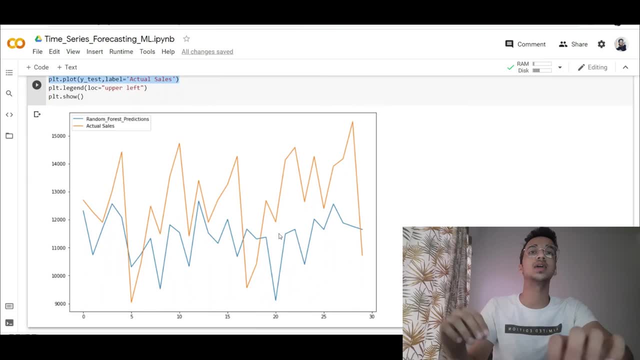 mentioning the figure size as 12 comma 8. so i'm going to basically plot the predictions and the actual test value and here is how the prediction is right, so you can see it's. it is still somewhat capturing the trend. now you can experiment. now i use only the past three months, right, you can experiment with six. 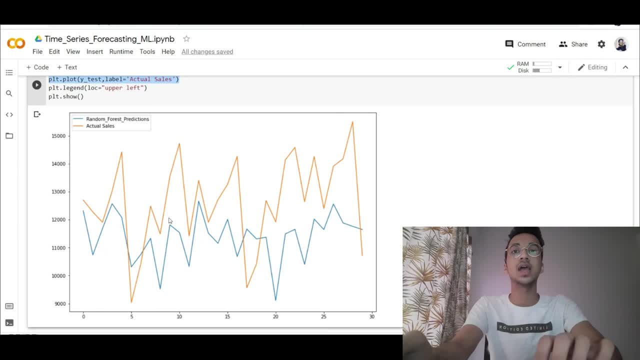 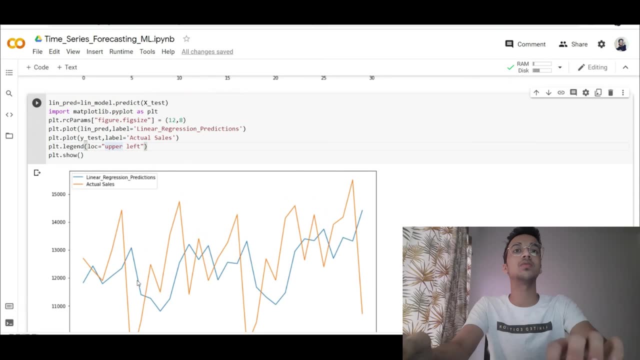 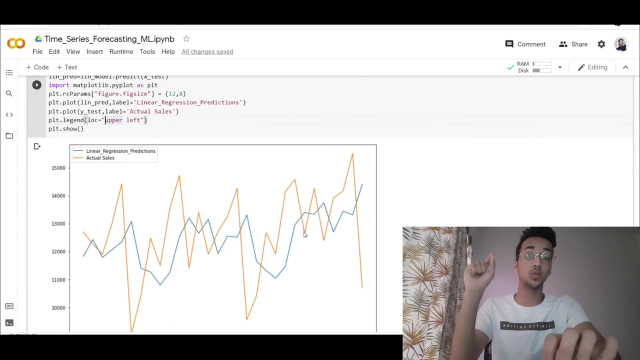 months or eight months, depending upon what kind of data set it is. and here is my linear regression models predictions and, as you can see, right, it captures the trend better. it right, because the actual sales and linear regression predictions are very close to each other, if you want to put. 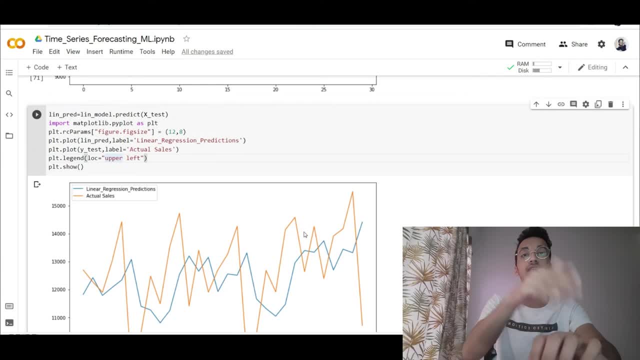 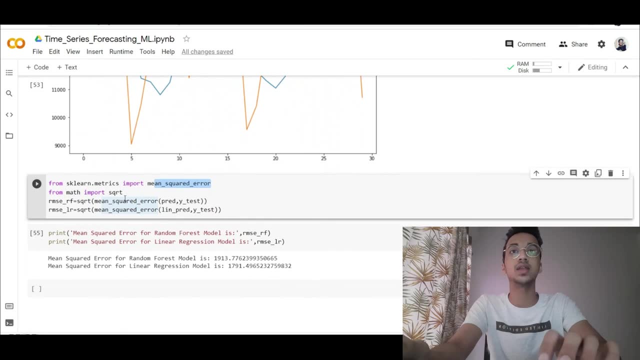 a number to that. we measure the mean squared error between the predictions and the actual values. so for that i import the mean squared error from skl, not matrix. and here is how i'm gonna do it. i'm gonna calculate the mean squared error, i'm gonna give it the predictions and the actual value and i'm gonna calculate square root of it. 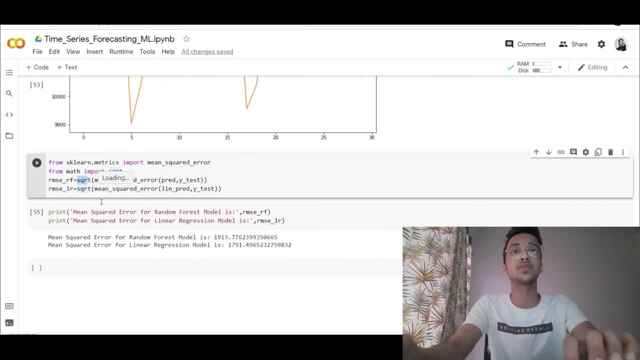 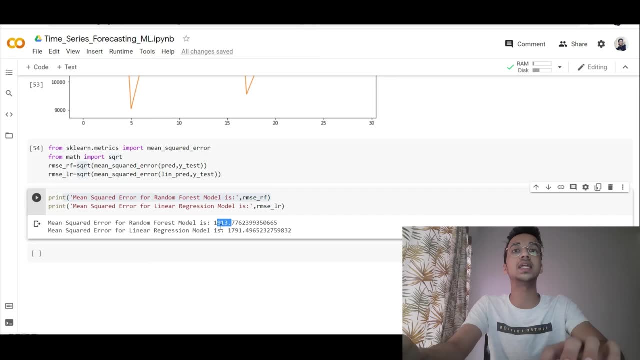 so it gives me the root mean squared error. so, as you can see, when i print these values for random forest- this is one for random forest it is 1913 and for linear regression model is 1791, so linear regression model performs better. so basically, you're free to use any kind of machine. 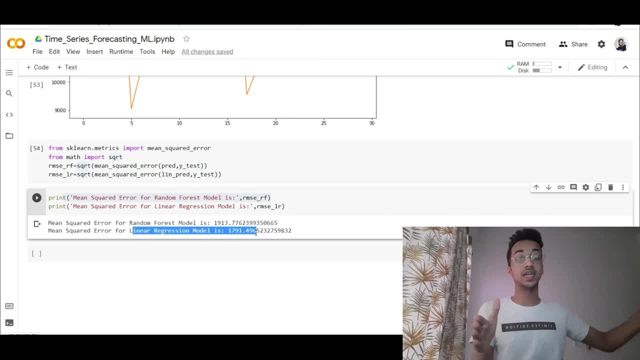 learning model you want and you can use more data from the previous time periods. you can also use other dependent variables. if i'm using sales in last month, maybe i can also use customers in last month or two months back or something like that. so basically, you just have to frame the data correctly. you have to have an input and output. 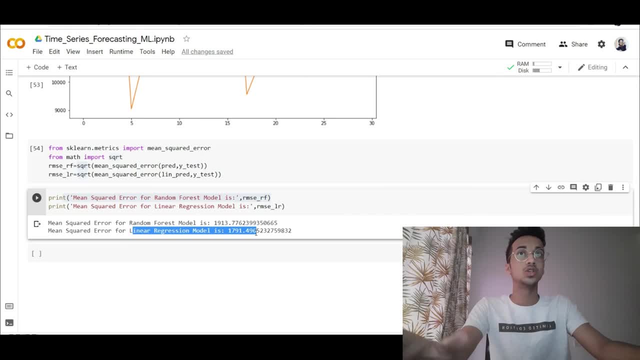 column and then you can use any machine learning model you want. so that was it for this video. i just wanted to bring this video to show you that supervised learning is also a good approach for time series forecasting in a lot of cases. so that was it for this video and if you did like it do. 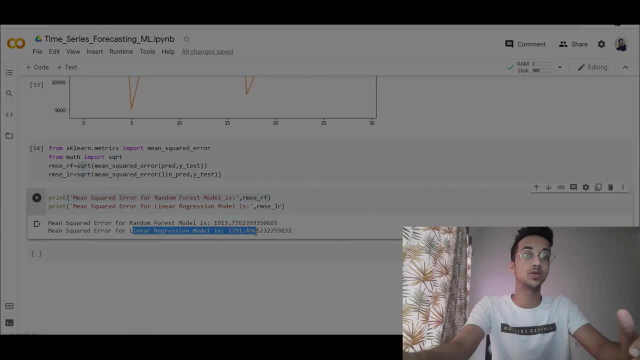 subscribe to this channel and like this video, and see you in the next video.